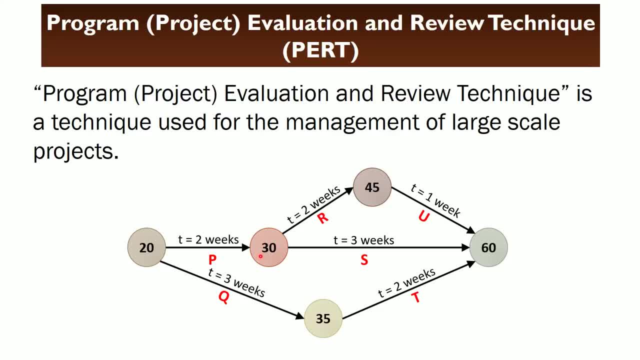 As you can see, a PERT chart indicates that prior to beginning a new activity, the predecessor activity must be accomplished. The milestones are numbered so that it can be easily understood that the last node has a higher number than that of the beginning node. 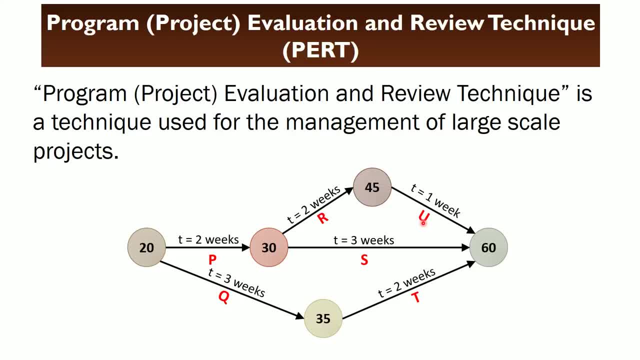 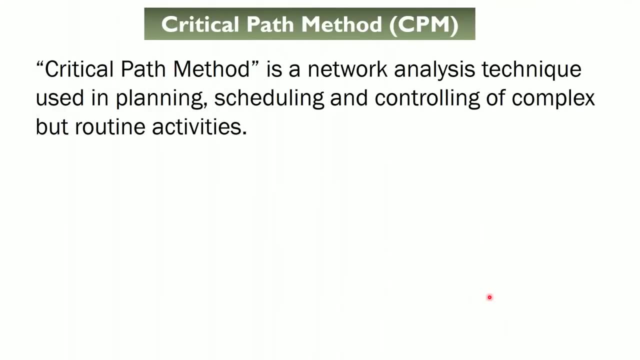 The activities are indicated by letters, Along with the expected time required for completing each activity. In this way, a graph can be plotted, and one can easily plan the activities involved in a project and estimate the time needed for its completion. Critical Path Method or CPM. 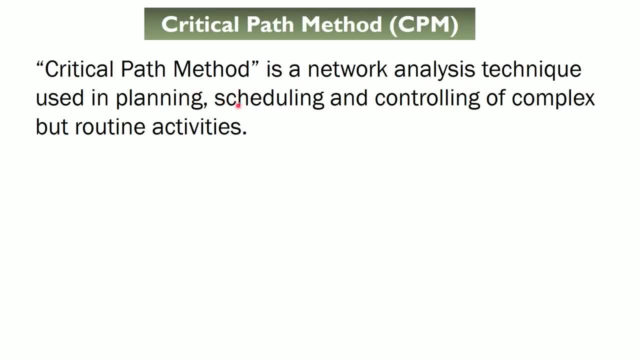 CPM is a network analysis technique used in planning, scheduling and controlling of complex but routine activities in a project. It is used to find out the earliest and latest activities in a project. It is used to find out the earliest and latest possible start time and finish time for each activity. 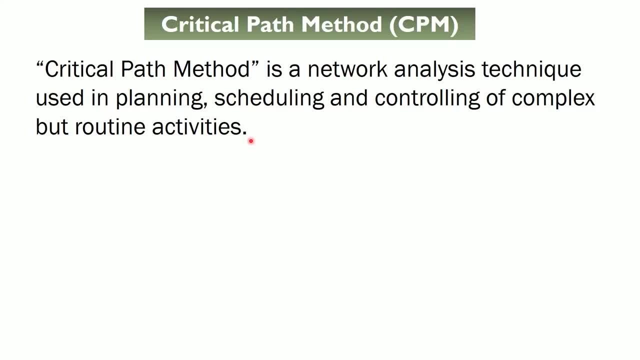 It is primarily employed in those projects whose time duration is certainly known, as well as the resources needed for completing the project is also supposed to be known. For this purpose, first of all, we need to identify the critical and non-critical activities on the basis of their importance to avoid chaos, queue generation and also reduce their time. 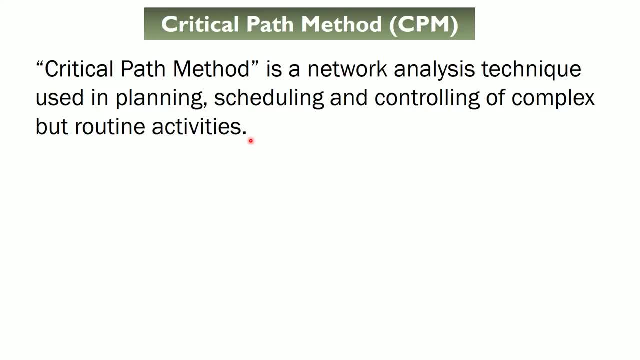 Once all the critical activities are identified, a network is drawn. This network connects all the crucial activities and shows which activity is to be carried out first so that the sequent activities can be performed successfully. This method is based on activity, on arc diagram to show critical path of activities, as you can see in the diagram here. 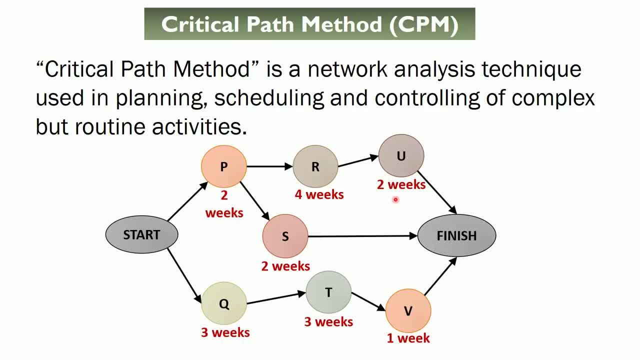 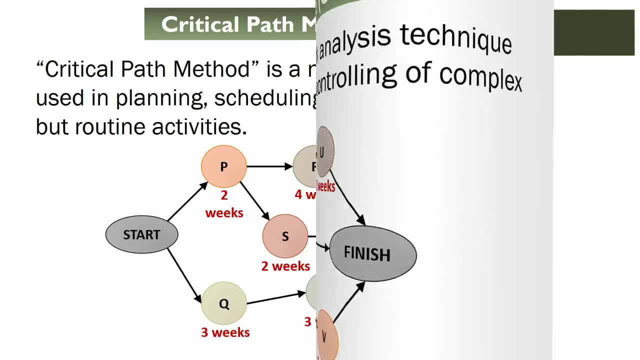 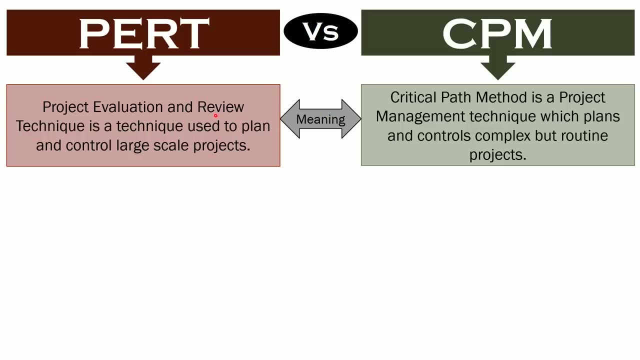 wherein the numbered nodes represent stages required for accomplishing the project, while arc represent the crucial activities required for completing the project, which are identified previously. Difference between PERT and CPM: PERT is a project management technique used to plan, schedule and control large-scale projects. 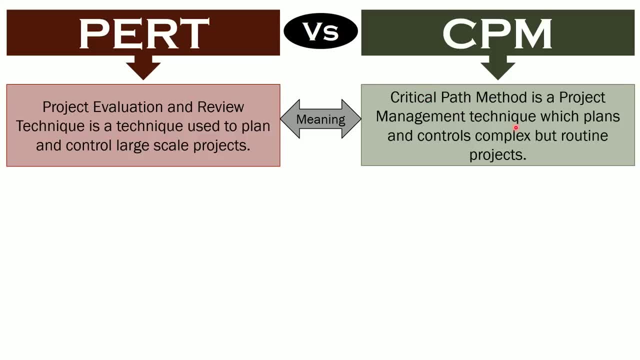 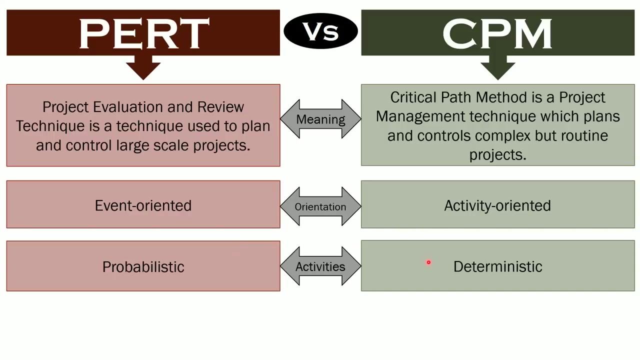 On the other hand, CPM is a project management technique which plans and controls complex but routine projects. In PERT network can be constructed on the basis of events, Whereas in CPM, jobs and activities forms the basis for constructing network. While PERT is based on probabilistic model, CPM uses a deterministic model. 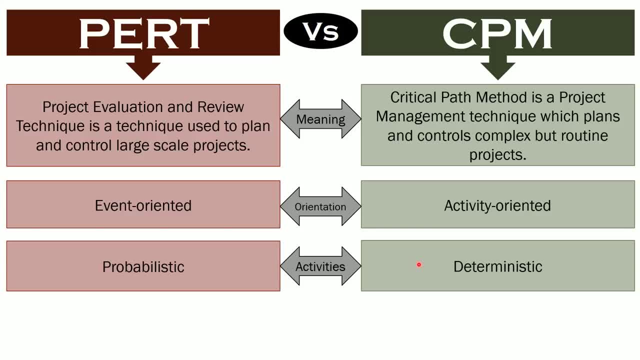 Because you can not identify how much time it will take to complete the project in case of PERT, But this is possible in CPM. When it comes to focus, PERT focuses on time, ie meeting time target or forecasting personnel Or forecasting percent completion. 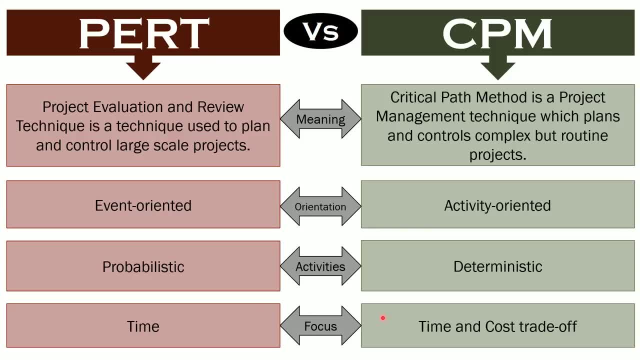 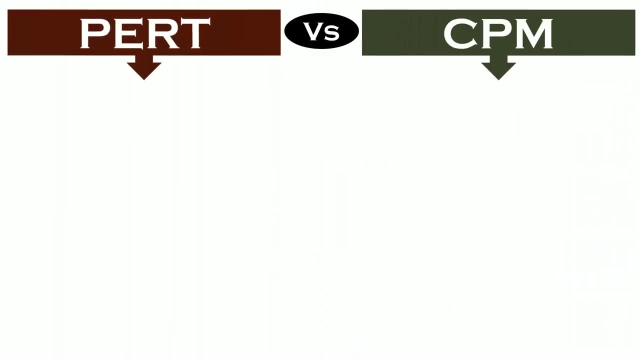 Conversely, CPM focuses on time and cost trade-off, As it gives importance to optimizing cost as well as crashing. concept can also be applied to minimize the overall project duration along with least additional cost. Next, While PERT is based on three times estimate, ie optimistic time, more likely time and pessimistic time- 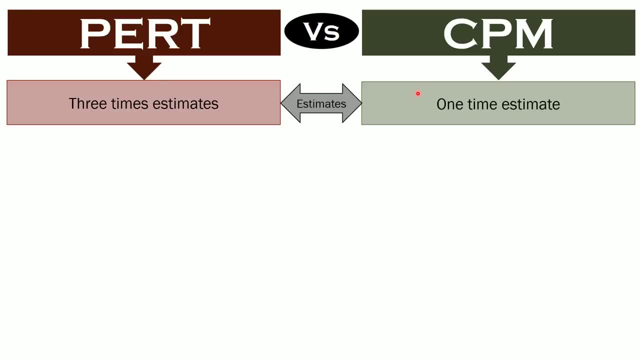 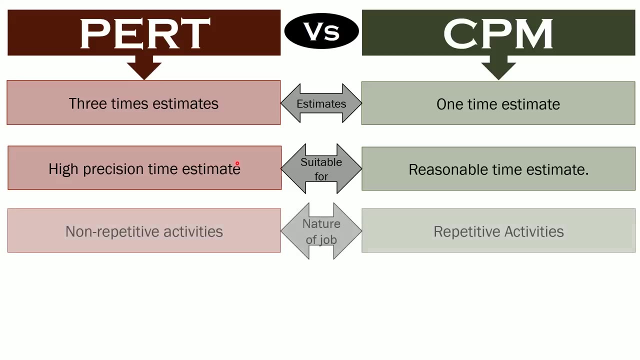 CPM is based on three times estimate, ie optimistic time, more likely time and pessimistic time, And based on single time estimate to complete a project. PERT is suitable for those projects which require high precision time estimate, Whereas CPM is best for those projects which require reasonable time estimate. 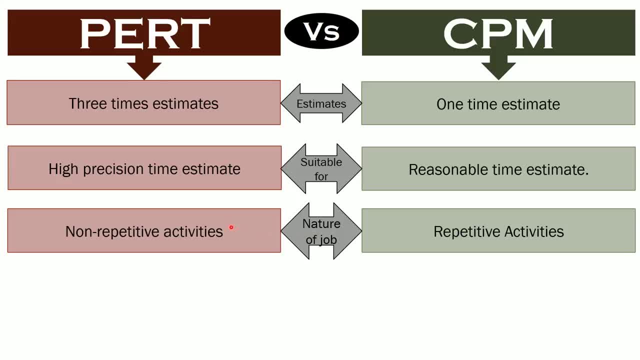 When it comes to nature of job, PERT is used where nature of job or activities is non-repetitive, Whereas CPM is used where nature of job or activities is repetitive. Lastly, PERT is mainly used in research and development projects because the activities are unpredictable in nature. 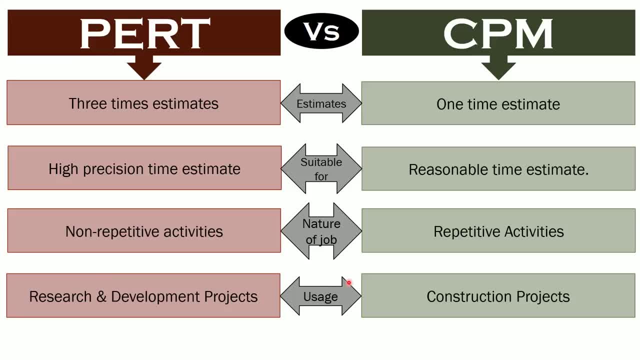 Whereas CPM is commonly used in construction projects, because here the activities are predictable in nature. Well, friends, this brings me to the end of this lesson. I hope you find the lesson very useful. I am sure that after watching this lesson, all your doubts regarding the difference between PERT and CPM are cleared now.